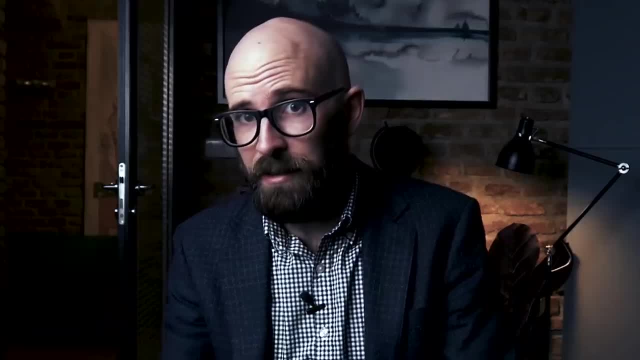 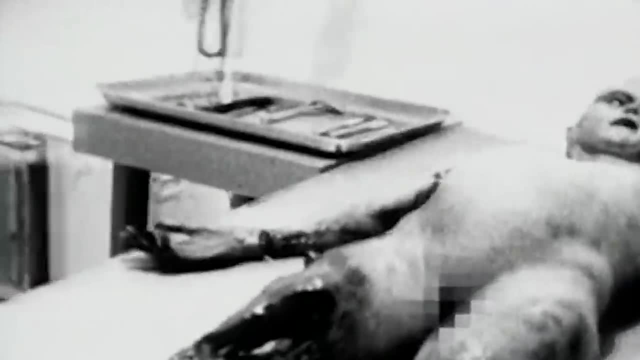 tends to draw the extremes of both sides. Some believe vehemently that there is in fact life out there and that we have already been visited by such beings: Roswell, Area 51, Little Green Men and, of course, anal probes, The myths surrounding our alien visitors. 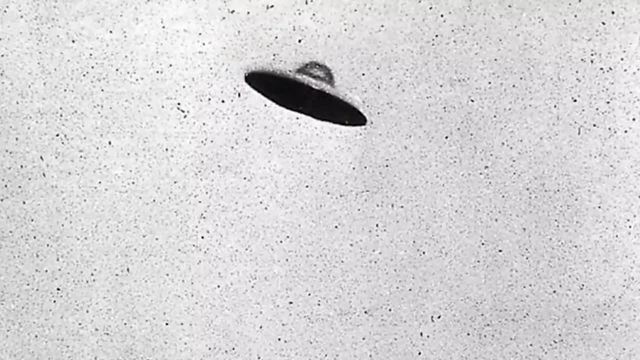 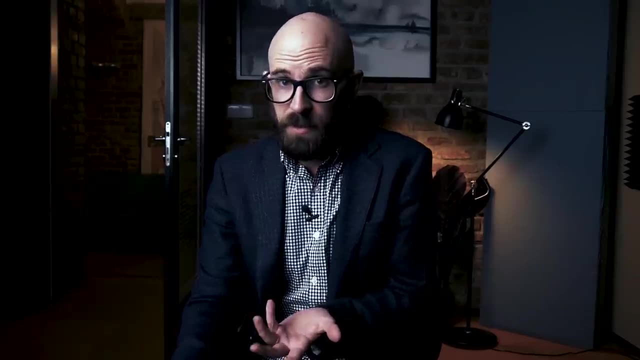 are tantalizing and definitely not proven. But to many it's not simply a question of if there are extraterrestrial beings, it's just a matter of where they are. On the other hand, some find the notion of extraterrestrial life absurd. It's placed in the same box. 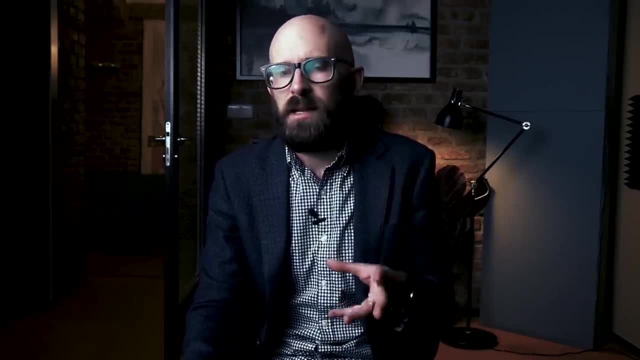 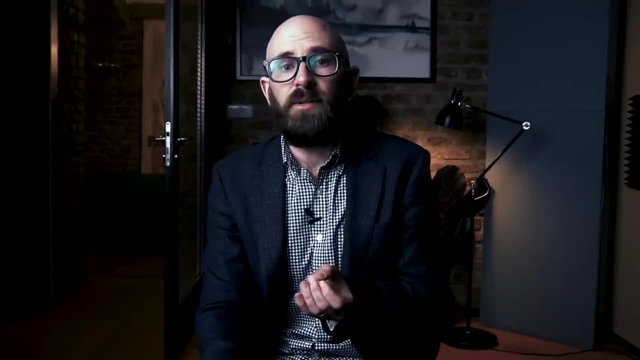 as ghosts, vampires and werewolves. Fun stories, but without any hope of being true. As I said, these are the extremes, But most people sit somewhere in the middle waiting for proof. We are, after all, not talking about man-made mythical stories. SETI is led by science and 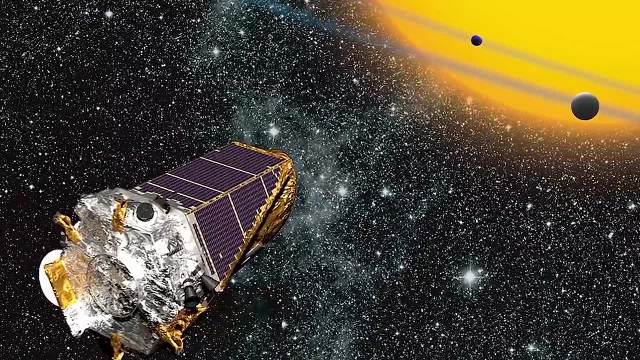 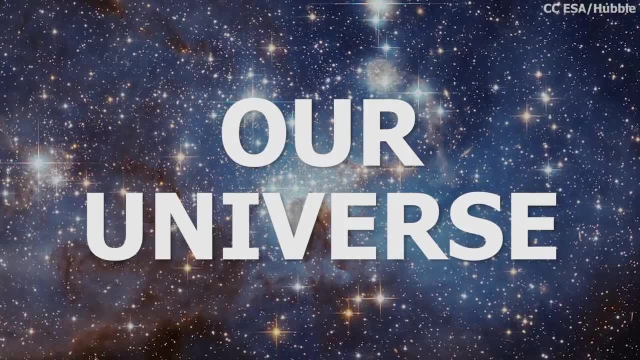 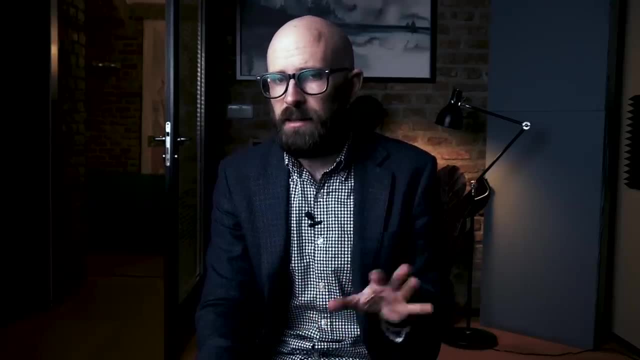 it's only through such science that we will ever be able to answer the question of whether we are alone in the universe. Scientists estimate that the number of potential planets that could harbor life is an extraordinary 100 billion give or take. This number is difficult for the human mind to imagine, even while gazing out on the surface of the universe. The number of planets that could harbor life is an extraordinary 100 billion give or take. This number is difficult for the human mind to imagine, even while gazing out on the surface of the universe, Even while gazing out on the surface of the universe. But how about the fact that the universe is probably in the region of 100 billion light years in diameter and that just one of those light years is the equivalent of 9.5 trillion kilometers? With such mind-bending sizes, it's not hard to understand why so much time and effort. 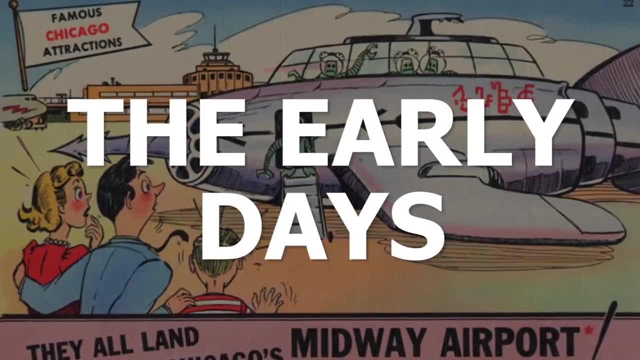 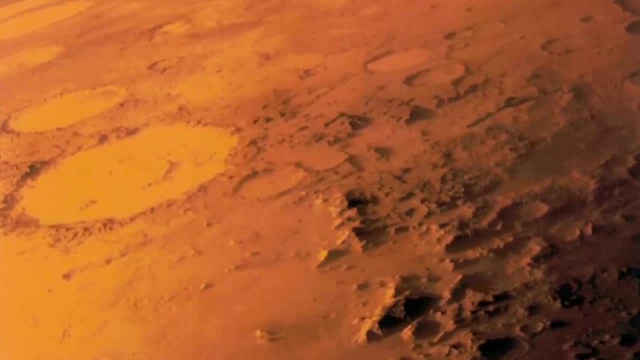 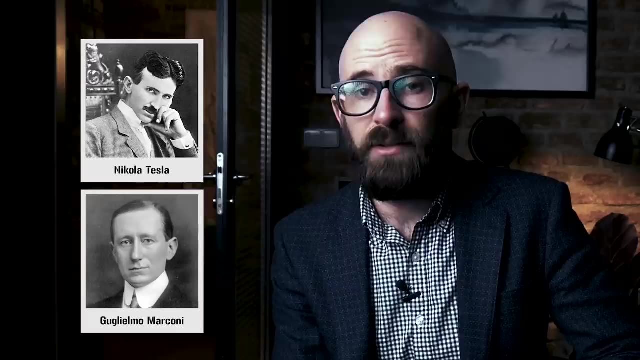 has been put into the search for extraterrestrial life. In the late 19th and early 20th centuries, much of the attention fell on our neighboring red planet, Mars. Tesla, Peter Marconi Both believed that with the use of wireless electrical transmission, we should be able. 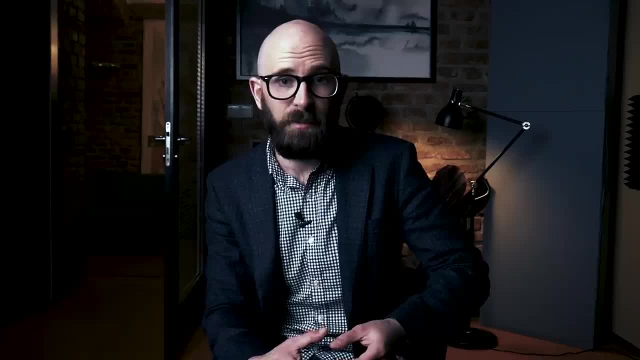 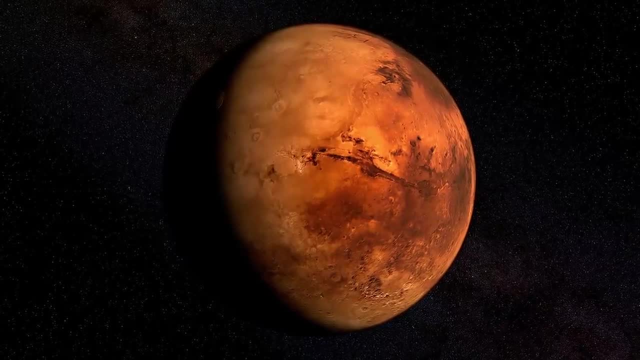 to speak with our Martian friends. Both, at one point, believed that they had picked up transmissions that could be from Mars, but obviously they weren't. Between the 21st and 23rd of August 1924, Mars moved closer to Earth than it had been. 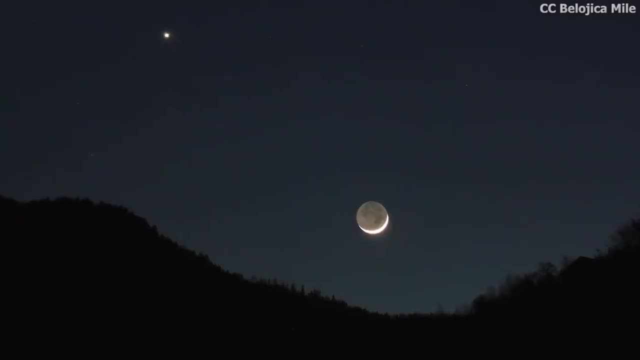 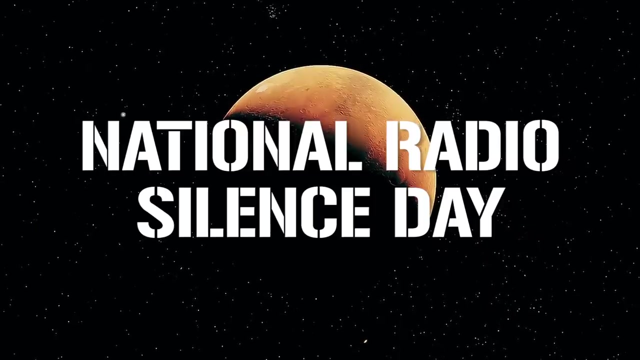 for around a century, and it wouldn't be that close again for the next 80 years, So surely this was the moment the Martians would contact us. An excited buzz rippled across America, and National Radio Silence Day was promoted across those days, with people encouraged to turn down their radios for five minutes at the 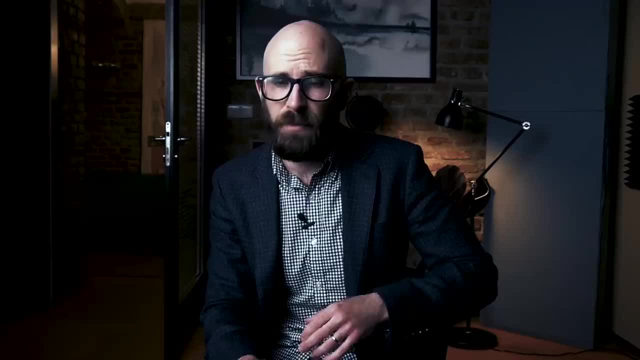 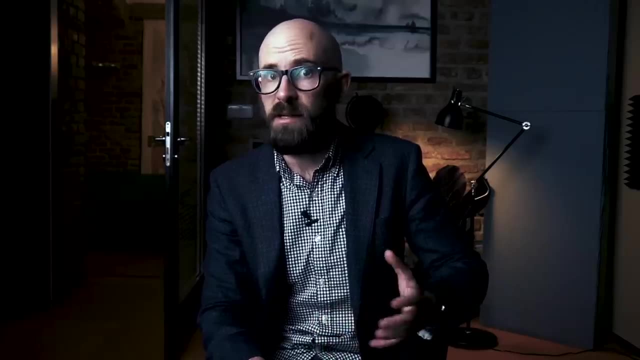 top of each hour. At the same time, a huge radio receiver attached to an airship was lifted three kilometers above the United States Naval Observatory in Arizona, where it waited expectantly. To give you an idea of just how seriously this was all taken, the head cryptographer. 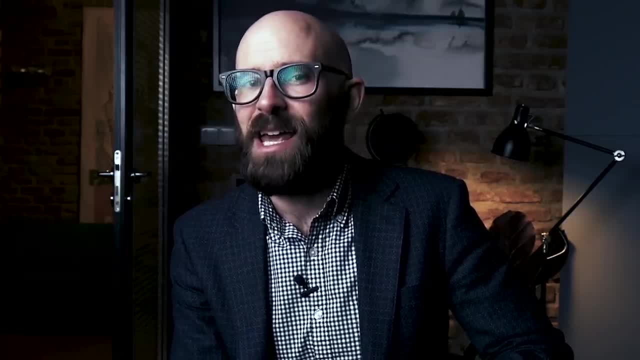 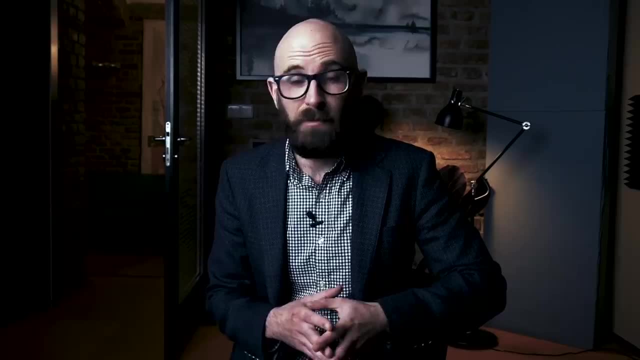 of the United States Army was waiting at the ready to translate any potential Martian messages. If this sounds a little rudimentary, things picked up in 1960 with what we would consider the first modern SETI experiment. The first modern SETI experiment. 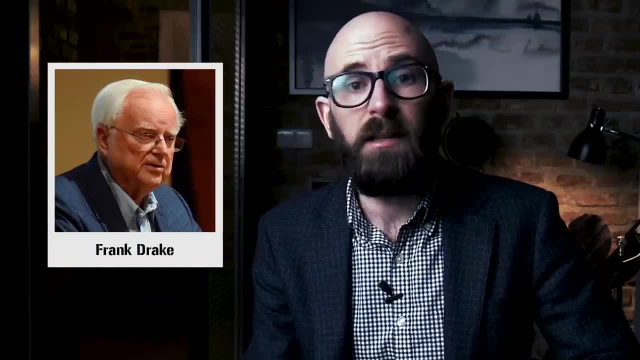 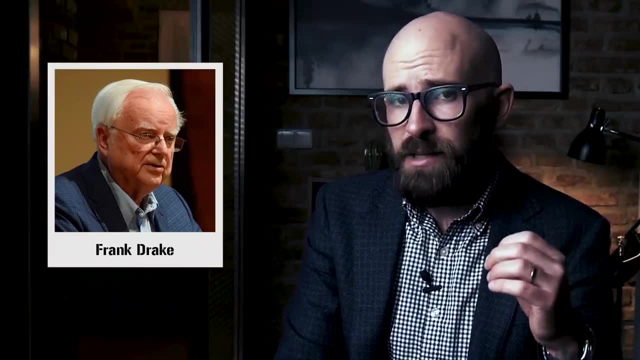 Project OSMER was carried out by astronomer Frank Drake in conjunction with Cornell University and was the first time distant planetary systems had been studied through interstellar radio waves With the help of a telescope measuring 26 meters in diameter. Drake focused his attention. 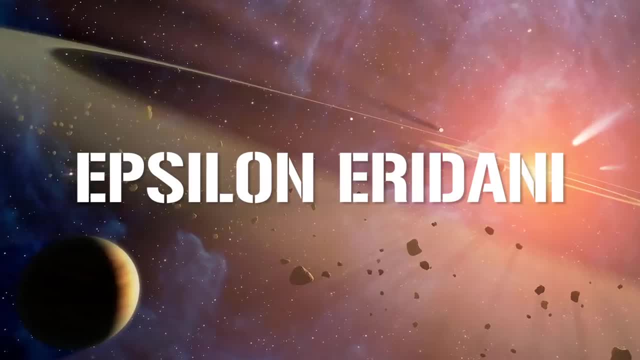 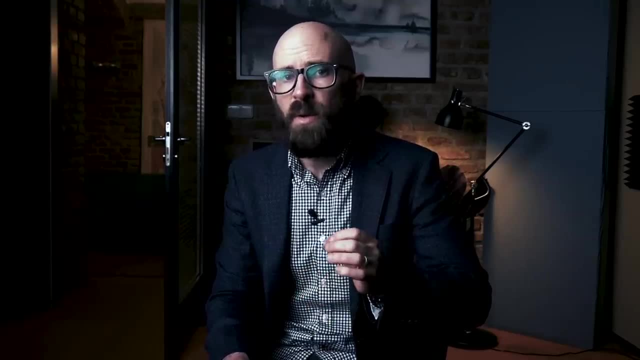 on two stars, Tau SETI and Epsilon Eridani, near the 1,420 GHz marker frequency, a quiet section of the electromagnetic spectrum known as the waterhole A 400 kilohertz band was scanned. This was the first time the SETI experiment had been carried out on an interstellar radio. 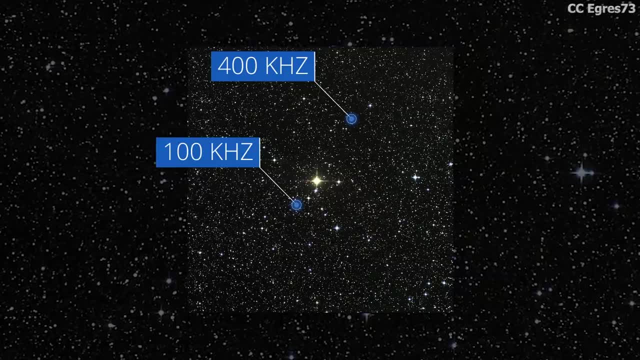 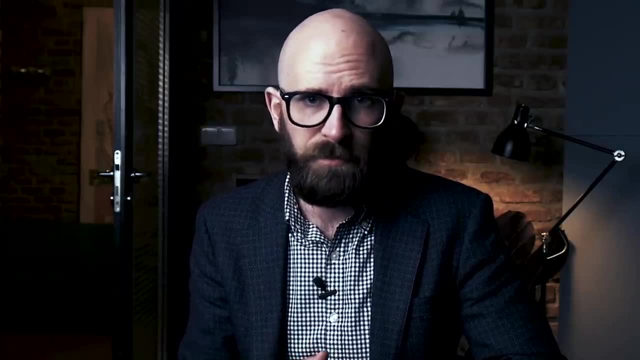 wave. It was scanned around this area with a single channel receiver at a bandwidth of 100 Hz. In total, 150 hours worth of recordings were taken over a four-month period that was analyzed after. Hans must have skipped a beat on the 8th of April 1960, when a signal was detected. 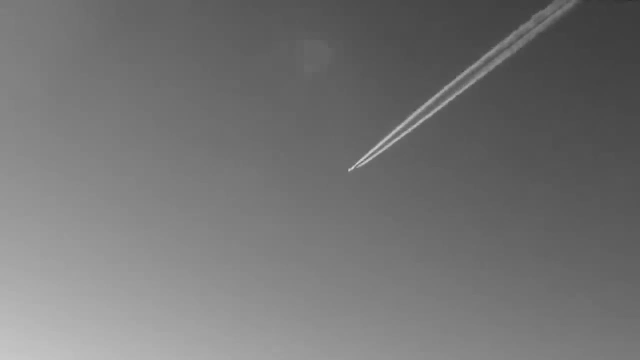 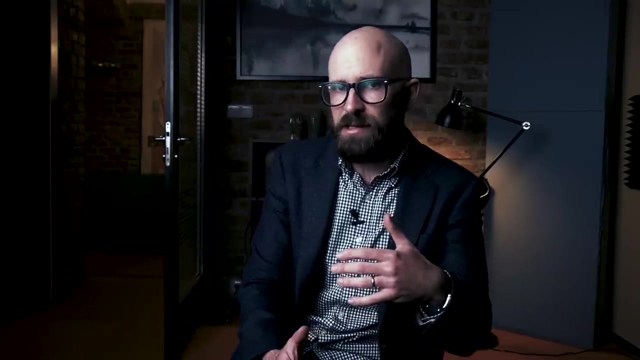 but this was soon deemed to be a false alert and perhaps it was just an aircraft traveling overhead. The Soviets also got in on the act during the 1960s and carried out numerous searches using omnidirectional antennas in the hope of picking up a signal, but it was definitely 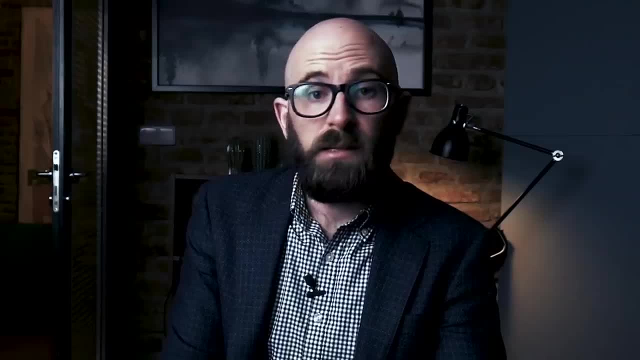 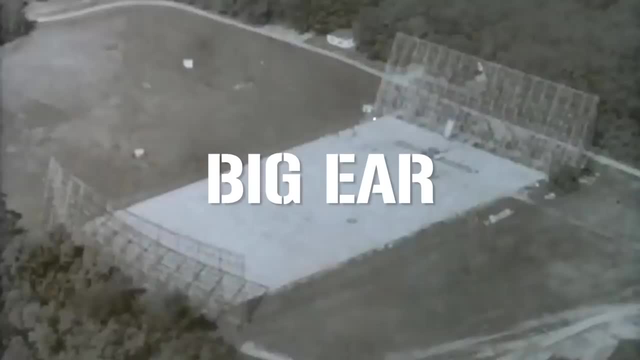 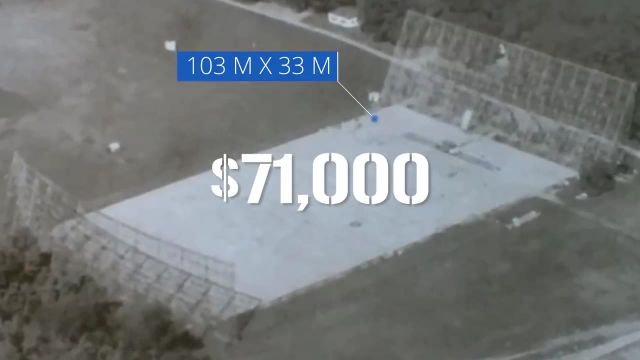 in the United States, The first formal continuous SETI program was established at Ohio State University, which began in 1963.. The radio telescope known as Big Ear measured 103 meters by 33 meters and was paid for with $71,000 in grants from the National Science Foundation. 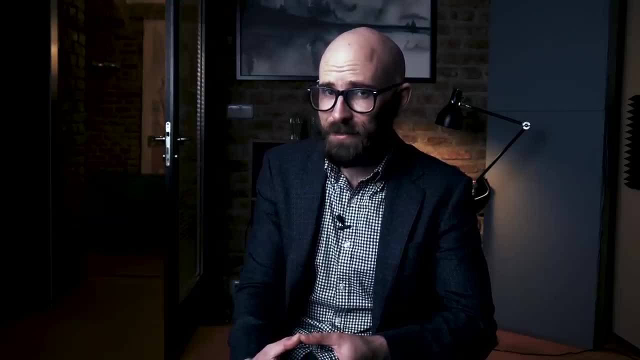 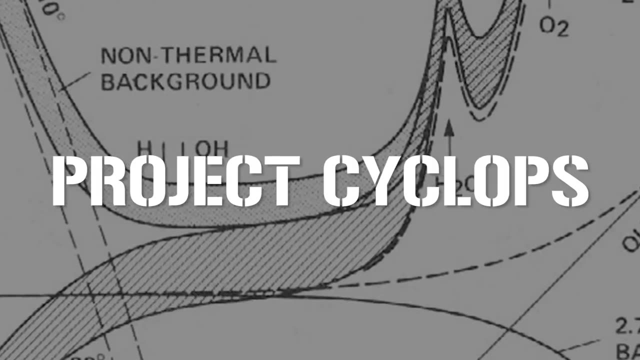 And, as we're about to come to Big Ear, definitely heard something. In 1971,, NASA commissioned its own SETI study, which came to be known as Project Cyclops. Though it was never started, the scale of it would have been a bit different. 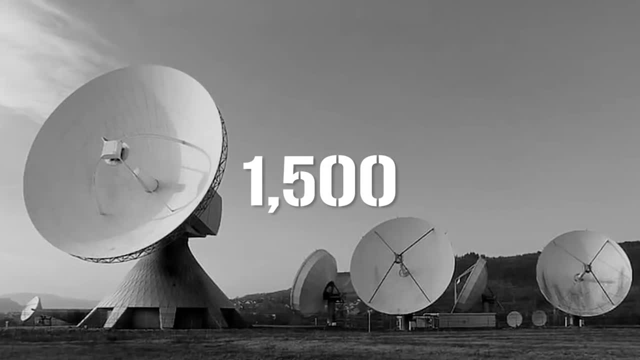 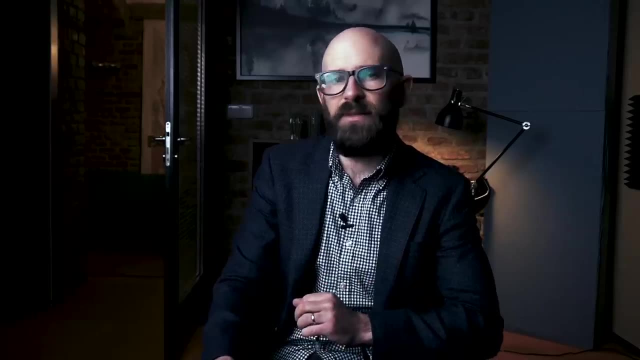 It would have been enormous, with 1,500 separate satellite dishes at an estimated cost of $10 billion, which is about $67 billion today. Project Cyclops never saw the light of day, but the framework would go on to be applied. 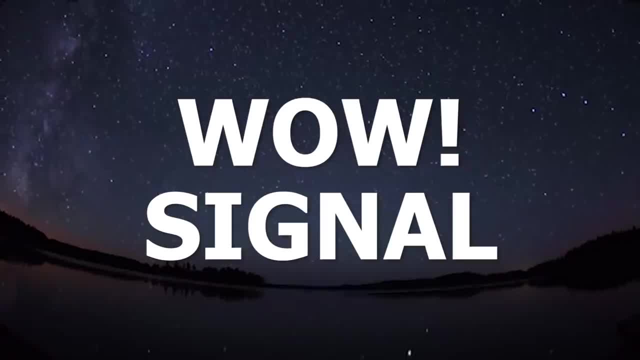 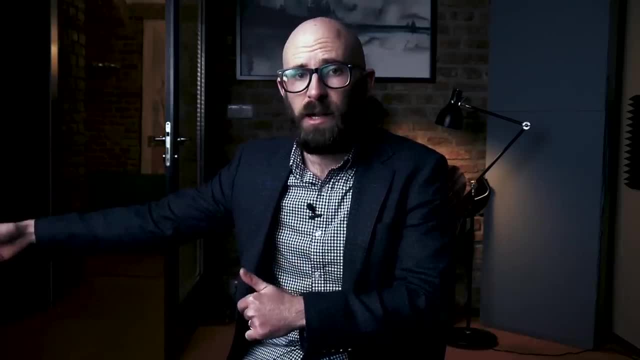 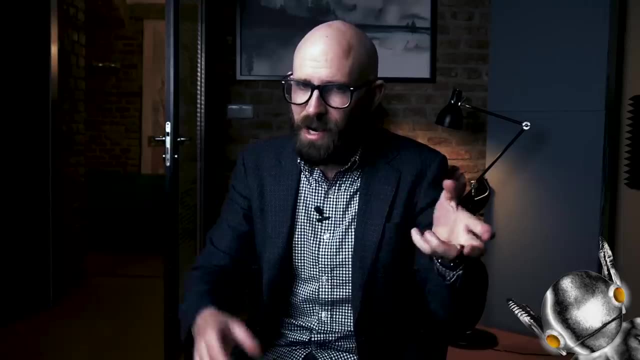 to future SETI programs. Okay, let's get back to Ohio State and the Big Ear Radio Telescope. Now, watching a video about the search for extraterrestrial life can be a little frustrating, for the quite obvious reason that we've never actually found anything. 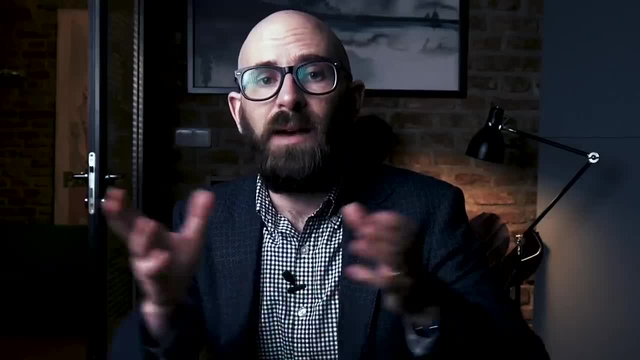 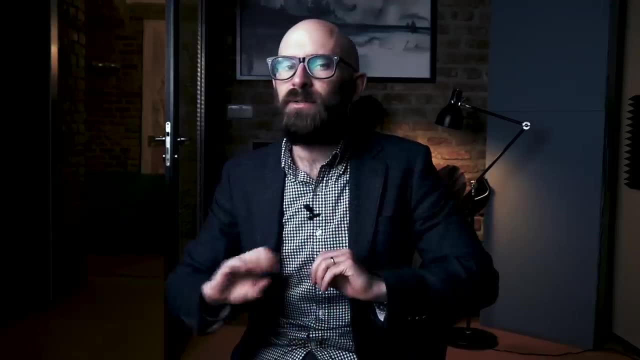 And we all know that. If you're expecting me to announce at the end of this video that we have in fact discovered aliens, well, spoiler alert, I'm not going to do that. No one really expected this, But occasionally the universe throws out a small glimmer of hope, and that was exactly. 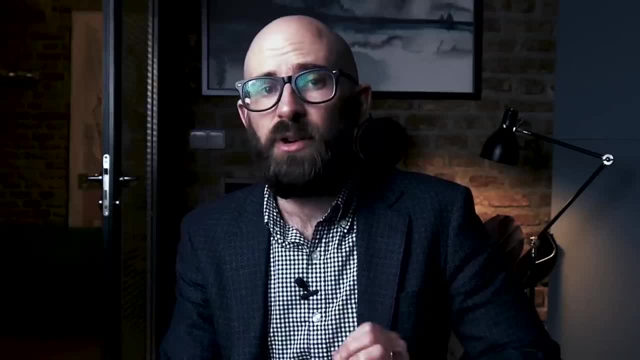 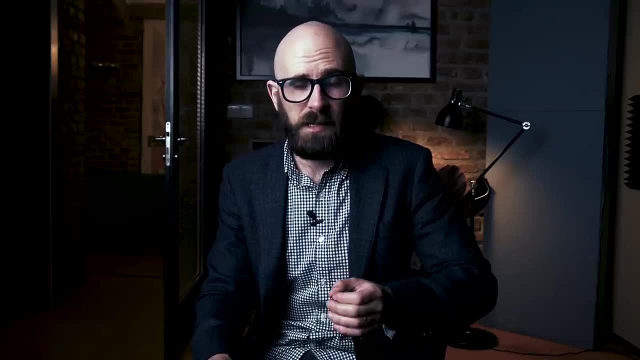 what happened on the 15th of August 1977.. A few days later, astronomer Jerry R Emin was going over the recorded data when he discovered something extraordinary Among the ones, twos and threes scattered around the page…. 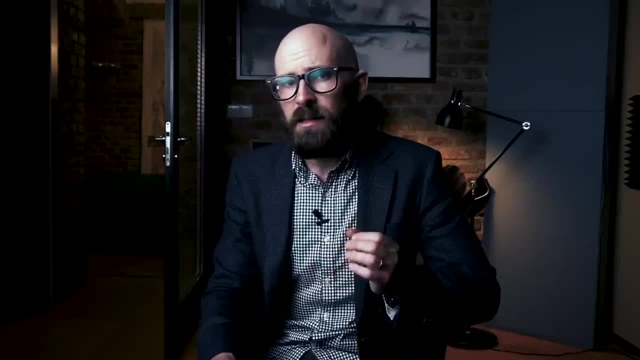 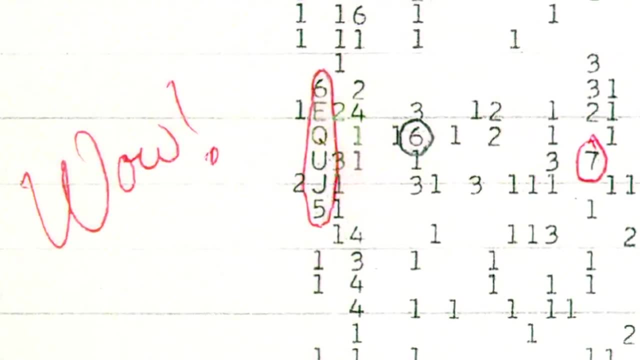 which represented the chaotic nature of radio signals. something appeared: 6EQUJ5.. This was not a message in itself, but rather an intensity variation over time. This six-digit form that had appeared in the computer readout represented a signal that 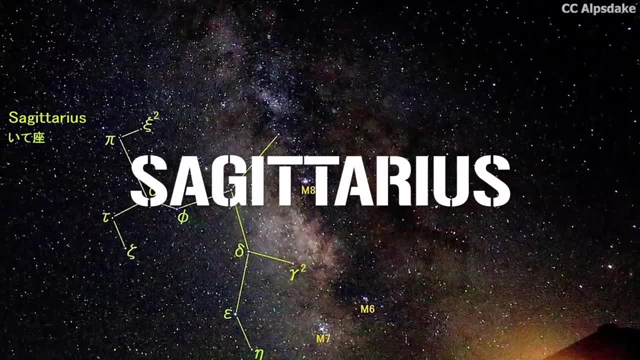 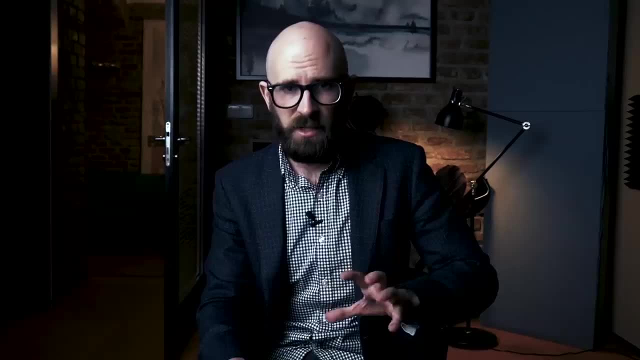 astronomers believed had come from the constellation Sagittarius, and what's more, it had lasted for the full 72 seconds that Big Ear was capable of observing it, for The telescope had a fixed position, so it relied on the orbit of the Earth to scan the 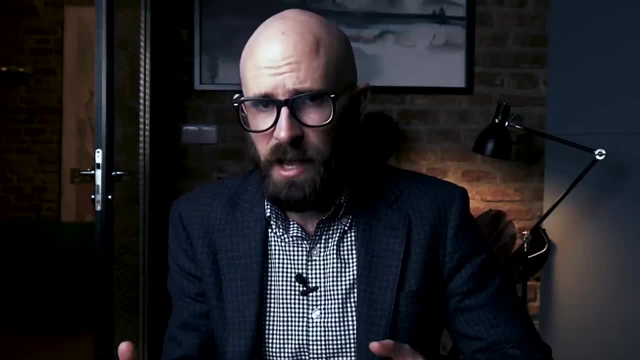 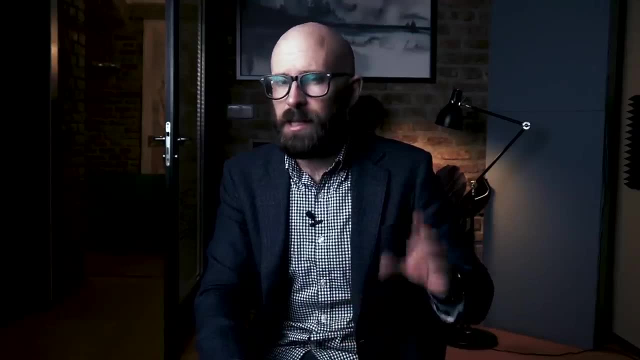 sky. So, whatever the signal was, it could have gone on for longer than 72 seconds. Emin scribbled WOW. next to it on the page and the name stuck. If you've never heard of this, it's probably because countless attempts to find the signal. 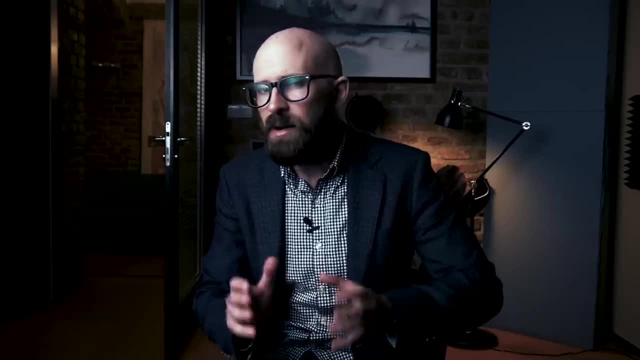 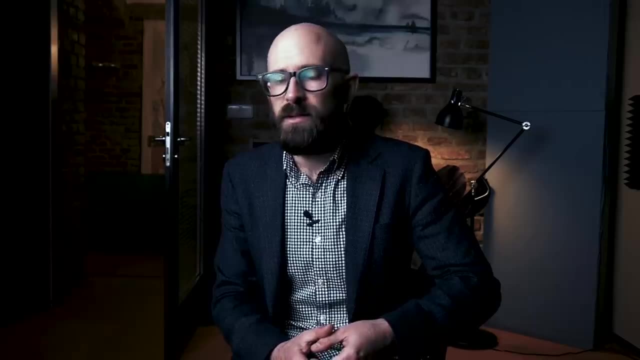 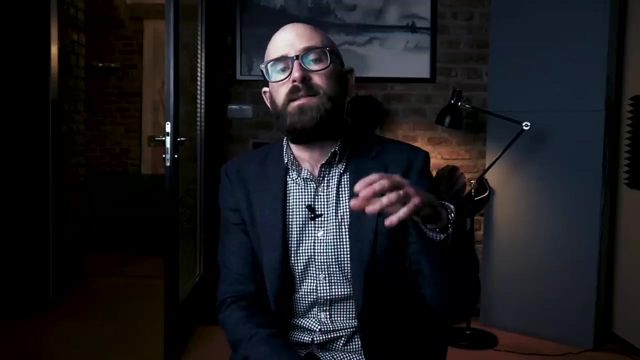 again have failed. Countless hypotheses were put forward, but no definite answer has ever been discovered And to this day it remains one of, if not the most likely, candidate for an extraterrestrial transmission: The Big Ear Transmission. The Big Ear Transmission, and in particular its Congress, made a habit of flip-flopping. 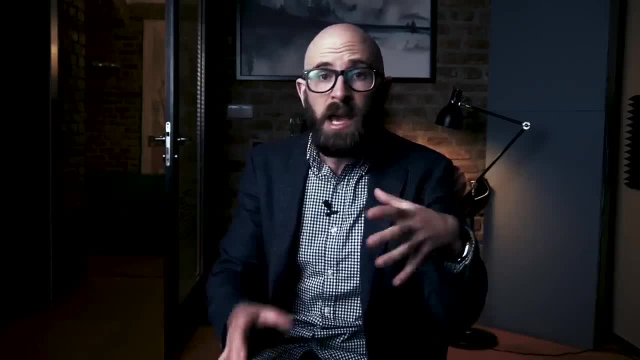 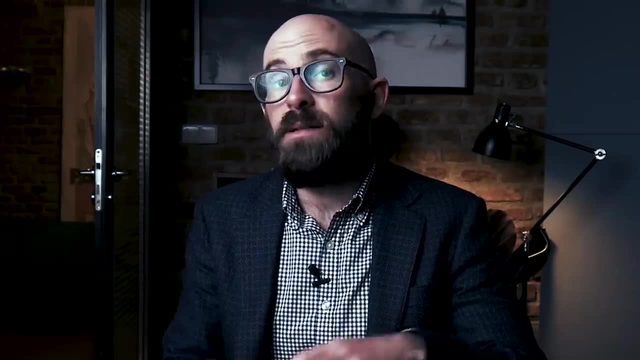 back and forth with SETI programs throughout the 1980s and 1990s. NASA's first serious SETI endeavor had a budget cut in 1981, only for it to be restored the following year In 1992,. however, things really got going with the Microwave Observing Program, MOP. 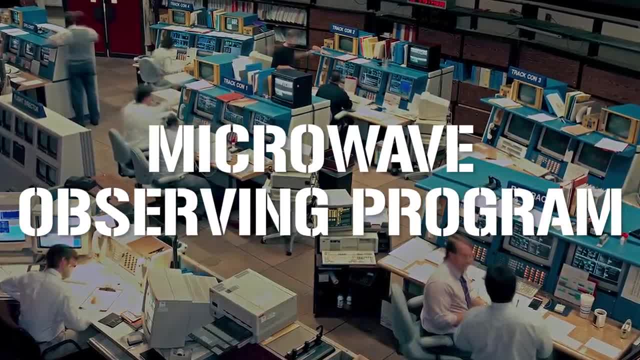 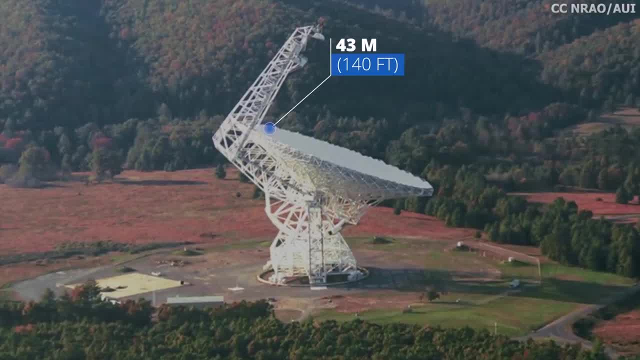 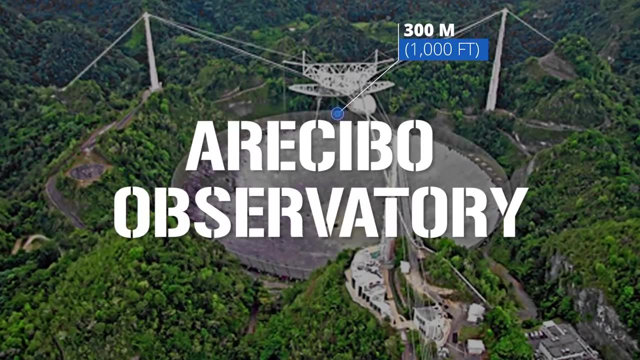 This would be a long-term survey that would carefully search 800 nearby stars using radio antennas used by the NASA Deep Space Network, as well as the 43-meter radio telescope of the National Radio Astronomy Observatory. The MOP would then be used to track radio signals gathered by all three using spectrum. 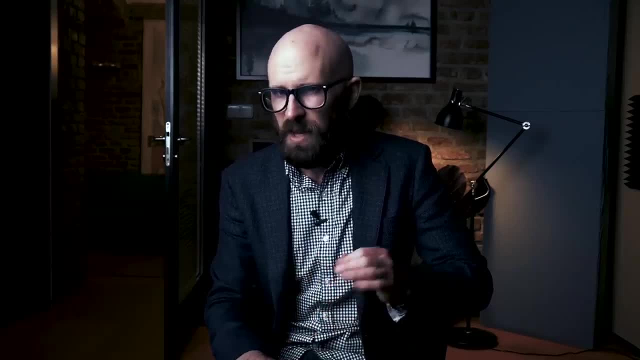 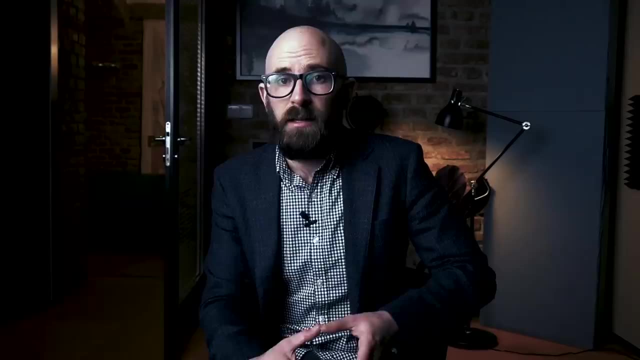 analyzers machines that could cover 15 million channels each. But just one year into the program it faced ridicule from within US Congress, with some viewing it as little more than a huge waste of money. Interestingly, many of the uber-religious congressional members within the House who have long believed. 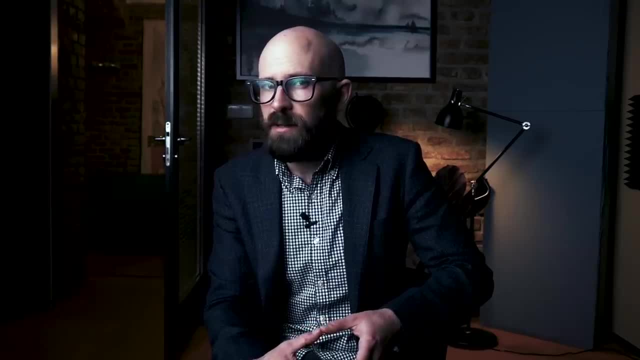 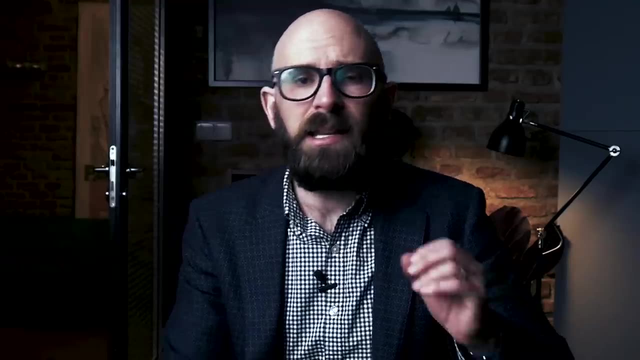 in an omnipotent presence above us, found the search for extraterrestrial life a little too hard to believe Really. But the program motored on without government funding and in 1995, the SETI Institute of Mountain View, California, essentially brought the entire program back to life. but this time under the name of Project Phoenix. As of 2012,, the yearly budget for the program was $2 million, with roughly 10 times that amount spent on all SETI programs around the world. There are countless SETI programs underway around the world and far too many to go into. 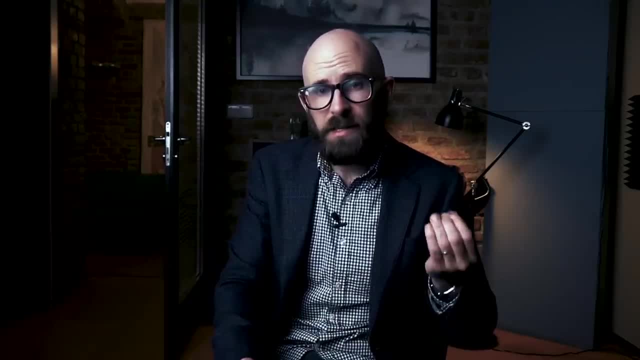 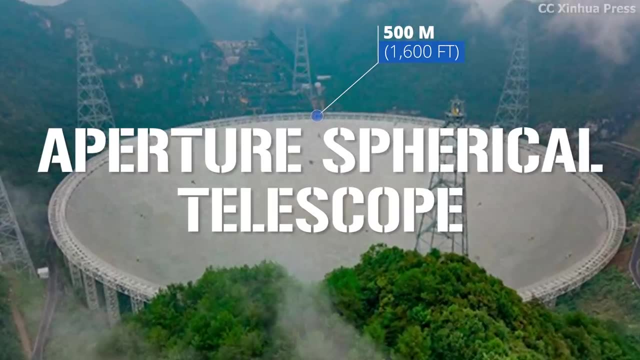 any great depth hereon. The world's first R&D program was the SETI Project. The first radio observatory built with SETI as a primary goal is China's enormous Aperture Spherical Telescope, which consists of a fixed 500-meter diameter spherical dish. Both Berkeley and UCLA universities in California have SETI programs, while Project Argus, which brings together a global network of amateur radio telescopes, falls under the SETI League, a non-profit organization set up in 1992 with 1,500 members across 62 countries. 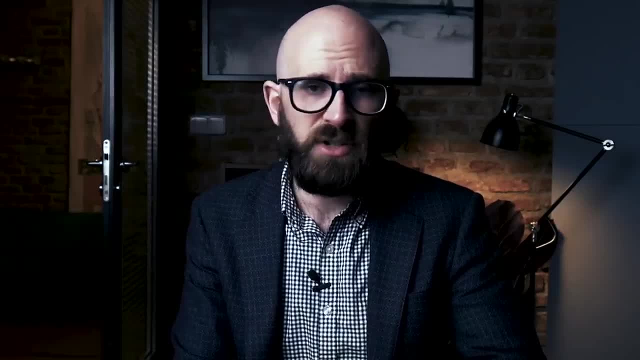 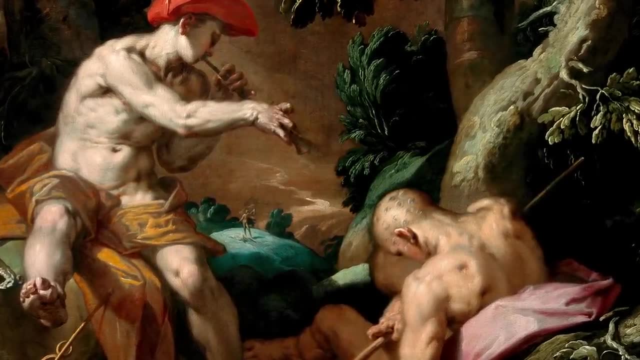 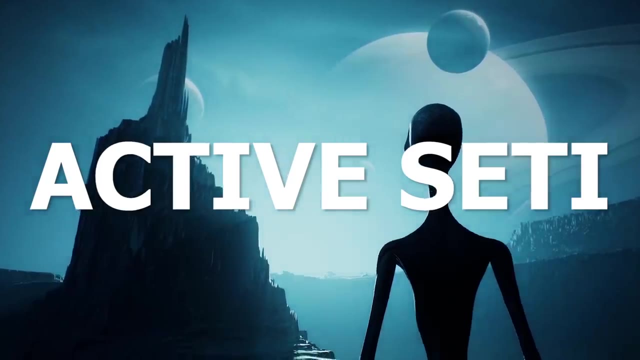 There are currently 143 Project Argus telescopes in operation in 2017.. If you're wondering about the name Argus, it comes from a mythical Greek beast who was said to have 100 eyes, so quite an appropriate name. SETI, While the majority of SETI programs have been 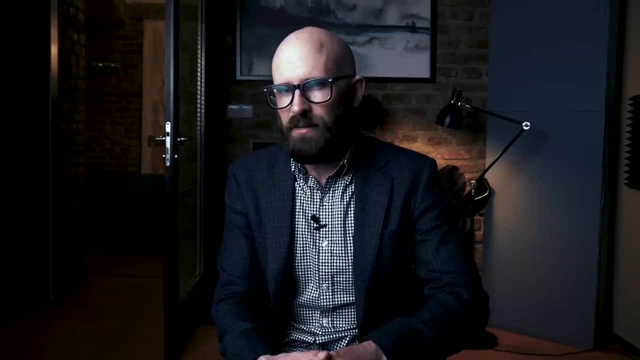 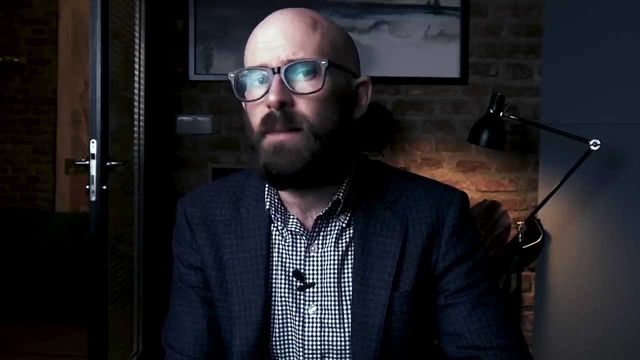 focused on monitoring radio signals. some have taken a much more active approach. Instead of hoping that aliens are sending signals to us, why not send signals out to anybody listening, Something that has come to be known as METI- Messaging to Extraterrestrial Intelligence? 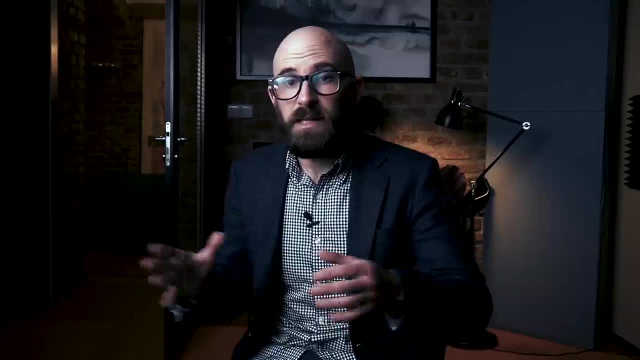 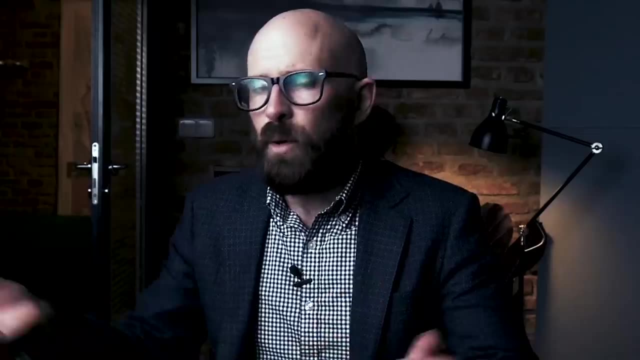 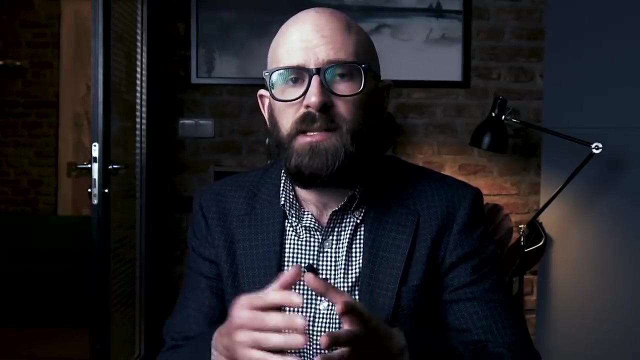 Sending messages out into space in the hope they might be picked up by somebody or something obviously comes with plenty of dilemmas. In what form do we send a signal? Words, Music, Images, They've all been considered. But even then, how can we be sure that whoever receives it knows how to interpret it? 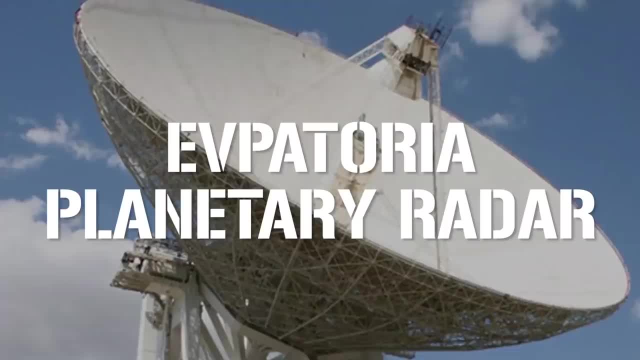 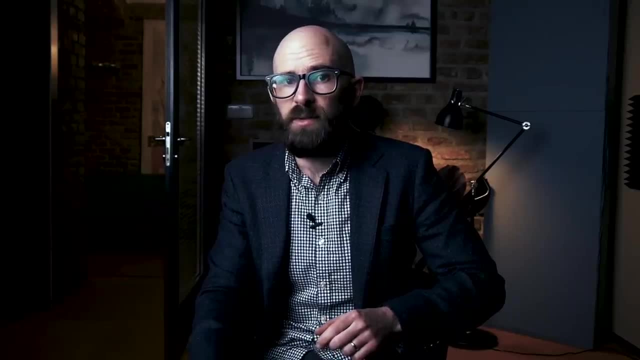 The first message to be sent was done through Morse code from the Aperture Planetary Radar in Crimea and directed towards Venus In typical Cold War style. The all-important message was Mir, meaning both peace and world. Lenin, CCCP. as in the 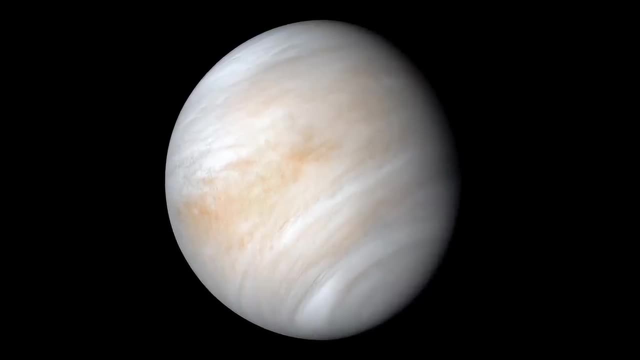 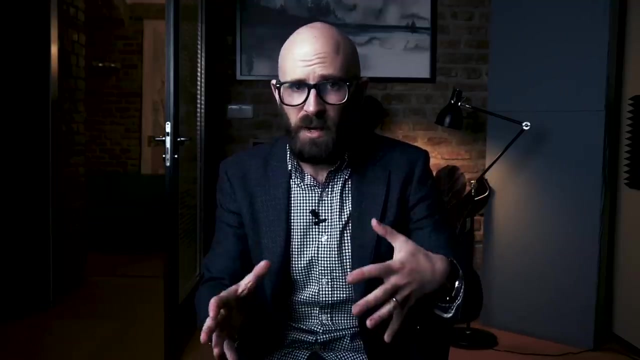 Russian spelling of USSR. Unfortunately, Venus never wrote back. Surprise. The Arecibo message, which left Earth in 1974, was a little more complex. The radio message consisted of seven parts that were designed to showcase human achievements rather than any meaningful attempt at communication. 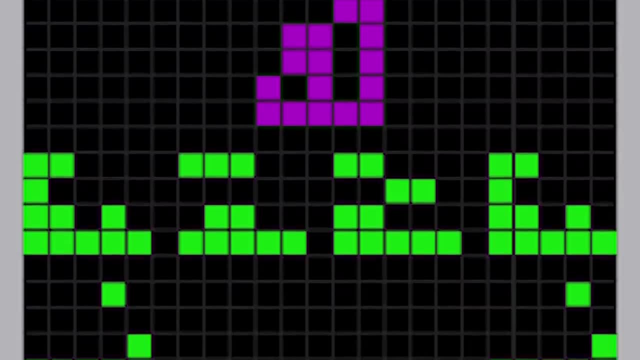 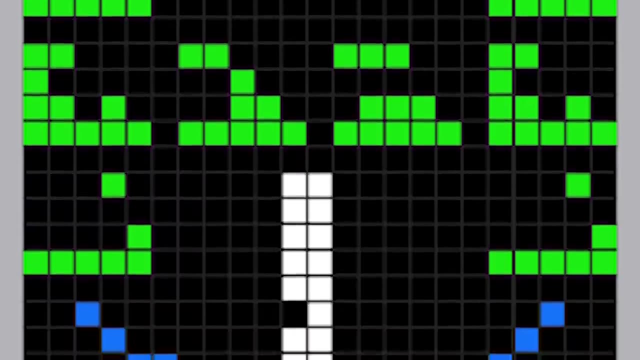 It included numbers from 1 to 10, atomic numbers of the elements hydrogen, carbon, nitrogen, oxygen and phosphorus Make up DNA, The formulas for the sugars and bases in the nucleotides, organic molecules of DNA, The number of nucleotides in DNA and the double helix structure of it. 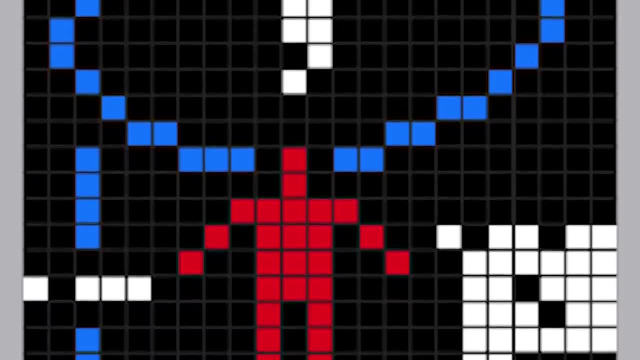 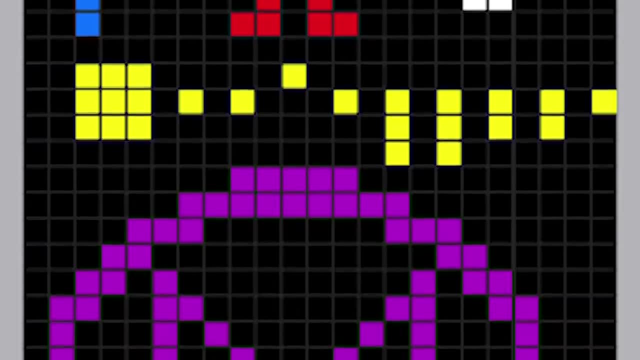 An image of a human, the physical height of an average man and the human population of Earth. An image of the solar system with a clear marker as to where the message had originated from. A graphic of the Arecibo radio telescope from where the message was beamed out from. 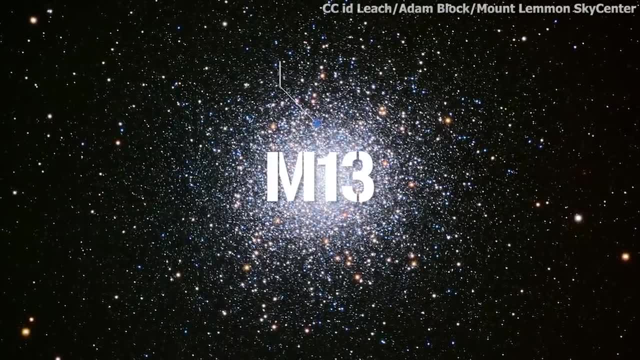 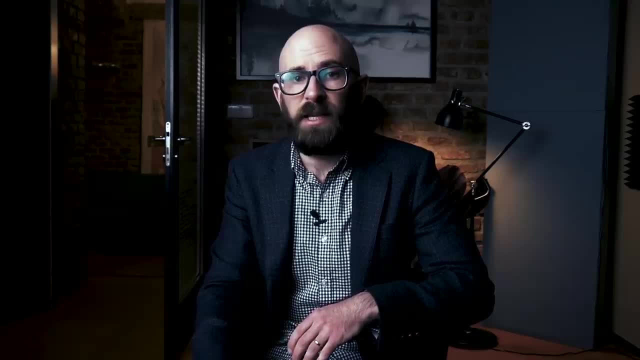 The message was directed at globular star cluster M13,, located around 25,000 light years away. There was, of course, no reply, but it did receive some fame when a hoax crop circle appeared in 2001 in the UK which copied the entire message in a field near the Chorbolton. 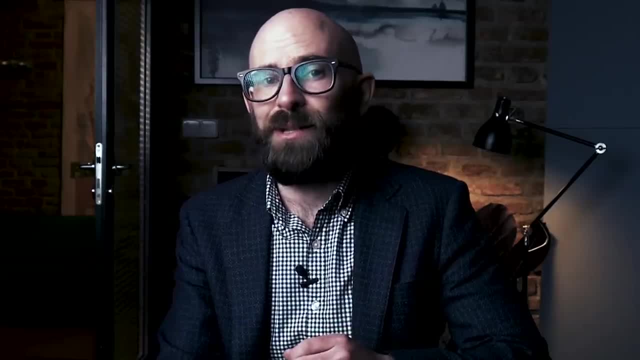 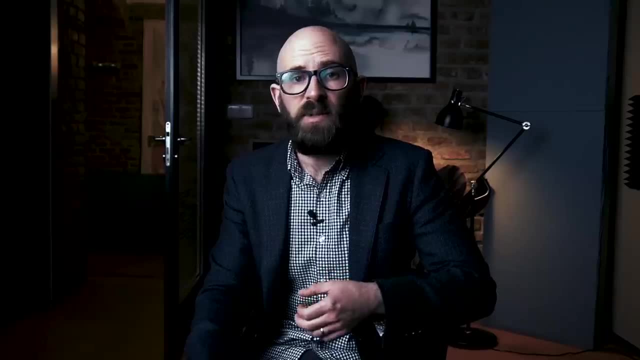 radio telescope in Hampshire In 2012,, a response to the WOW signal was sent that included 10,000 Twitter messages, as well as videos from various celebrities carrying individual messages. The most recent attempt was the sonar GJ237B, composed of 38 different 10-second pieces. 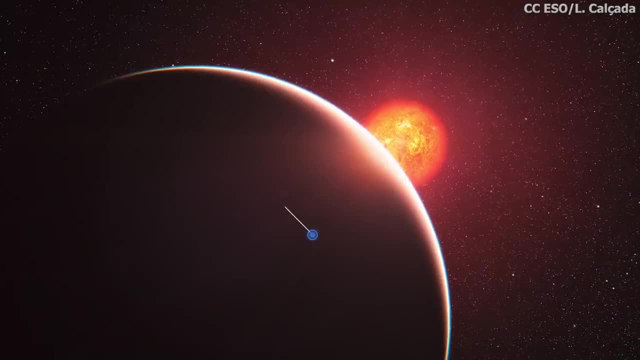 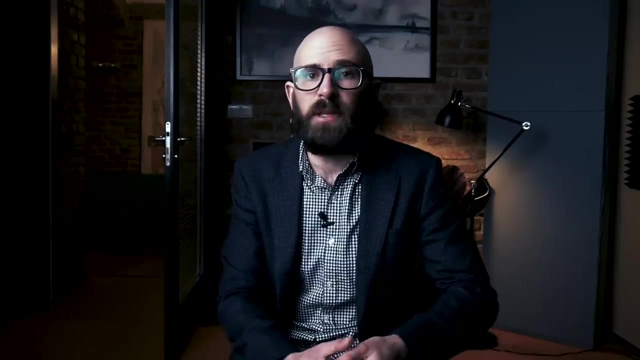 of music, each submitted by a different musician. The destination is an exoplanet 12.4 light years away. Scientists believe that at least it has the potential of being inhabited. The message is due to arrive at the planet on the 3rd of November 2030.. 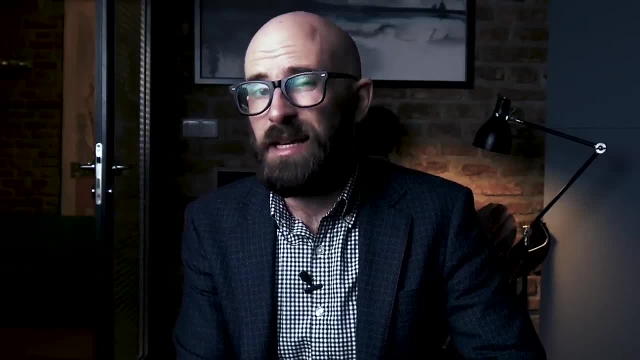 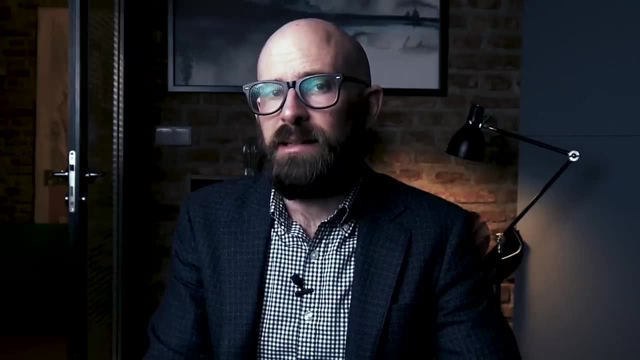 In total, 19 different messages have been sent out across the universe since the early 1960s. The practice has come in for some criticism because it tells the aliens: hey, we're here and they might not be friendly. One exciting idea that has been bandied around is the idea of a 10 billion watt interstellar. 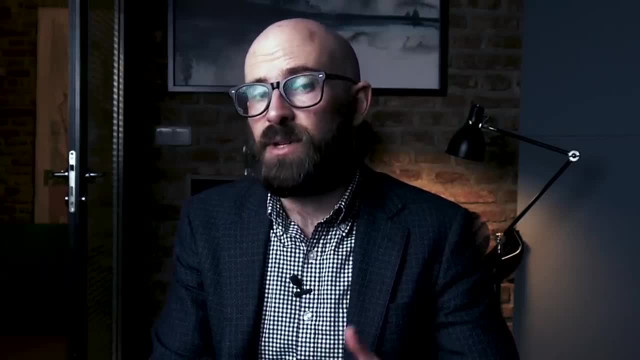 SETI beacon that would essentially send out millions of individual beams across the universe. When it was first put forward in the 1980s, it was thought to be a great idea, but it's been dismissed as being impossible. But scientists believe this could now happen. 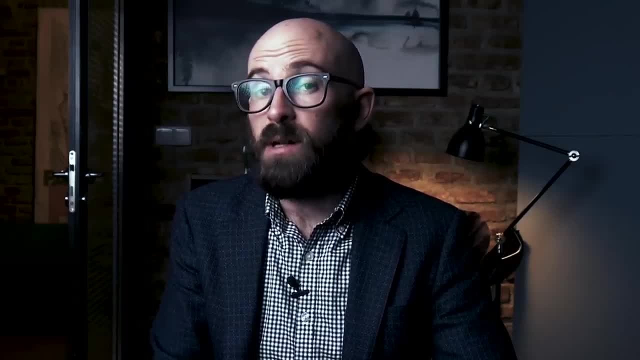 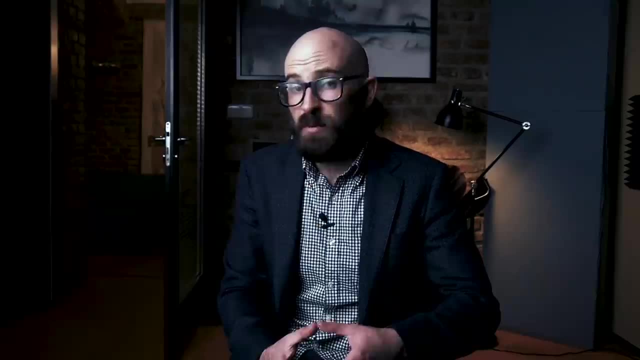 A study carried out in 2018 estimated that a 1.2 megawatt infrared laser beamed through a 30 to 45 meter telescope could be seen from as far away as 20,000 light years. Proponents of this idea say that once two civilizations have successfully found each